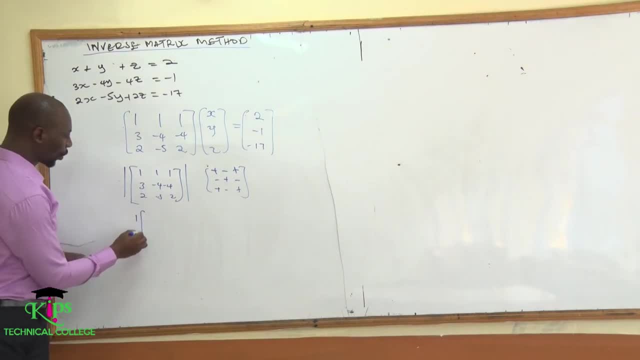 That one shall be one in two negative, four negative four negative five, two, Then minus one into three negative four, two, two, Then plus one into three negative four, two negative, five. By when you are at this point, you close this row and this column, you end up with this: two by two matrix. 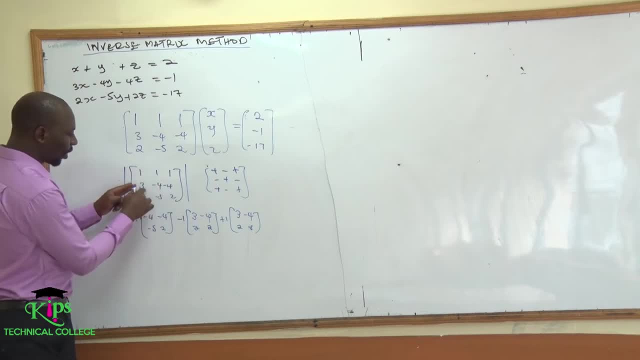 And when, at two, you close that first row and the middle column, you end up with this and this, this and this. So you just close the row and column where you are for you to be able to get the real matrix of the two by two matrix that you intend to get. 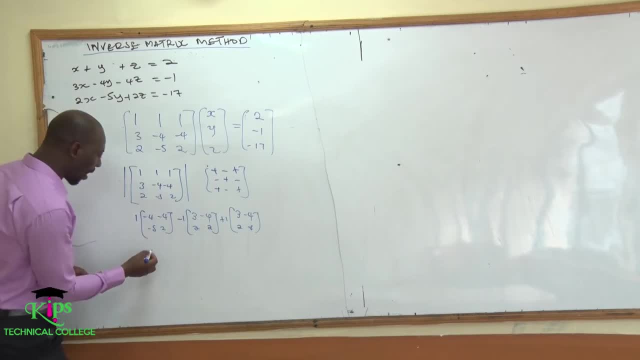 So if you get the the magnitude of this two by two matrix you shall have: this is negative eight minus twenty. negative one into six plus eight, Then plus one into negative fifteen plus eight, This one. if you solve all this one, you shall get negative forty-nine. 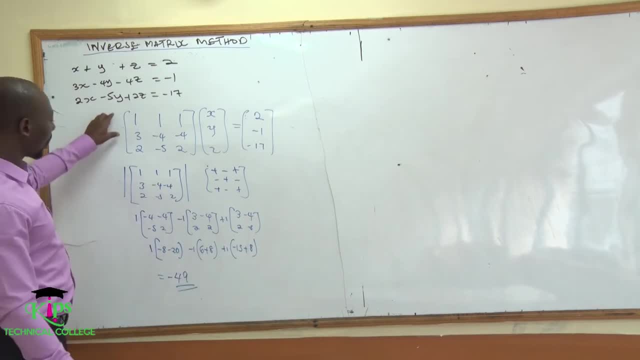 This one gives you Negative forty-nine. So the determinant of this three by three matrix is negative forty-nine. The determinant is negative forty-nine. The next step for you to be able to proceed so that you be able to solve for the inverse: 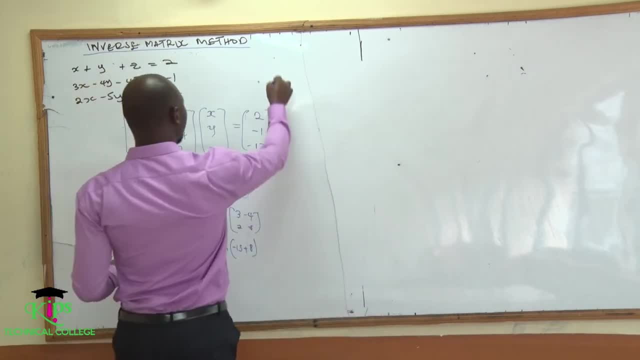 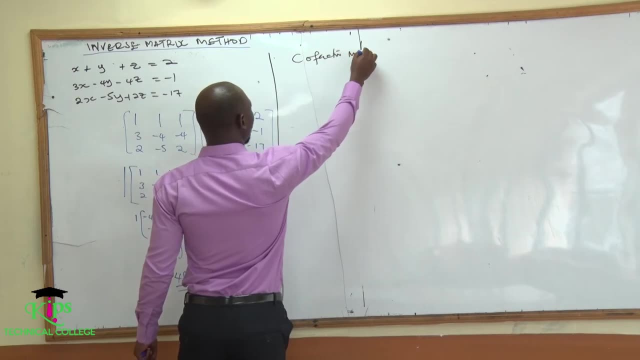 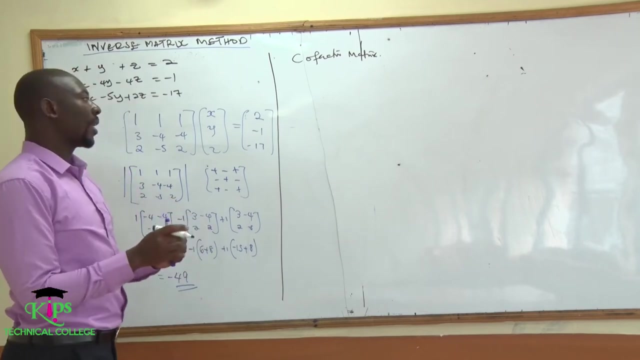 you form what we call a cofactor matrix. So the next step is to form a cofactor matrix. So let's form a cofactor matrix. The cofactor matrix is formed by taking two by two matrices at each and every point, then matched by the sign from the sign array. 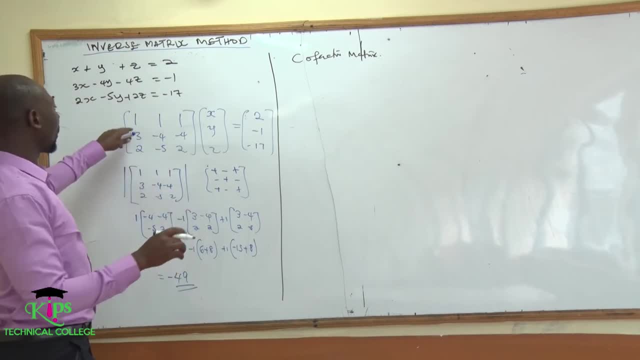 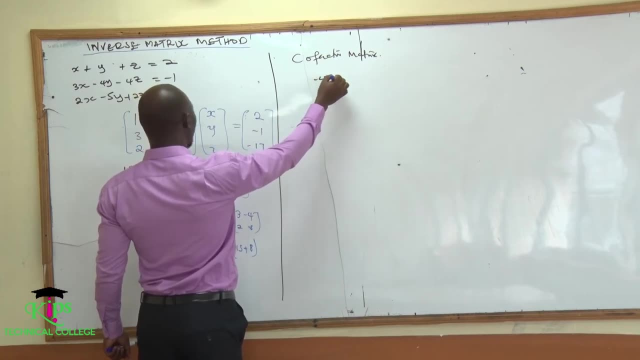 So let's have the two by two matrix from this one. So the first one. at this point you start at point one, you close the row and column, you remain with the two by two matrix. that is negative four, negative four. 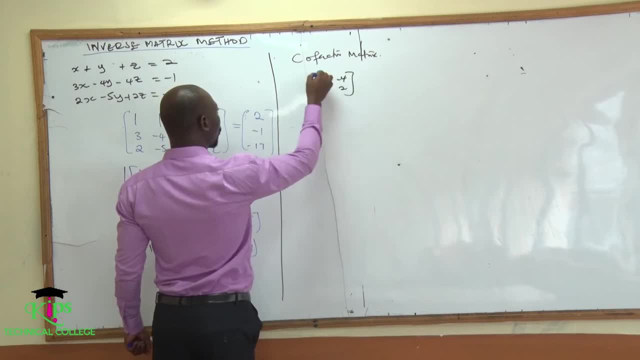 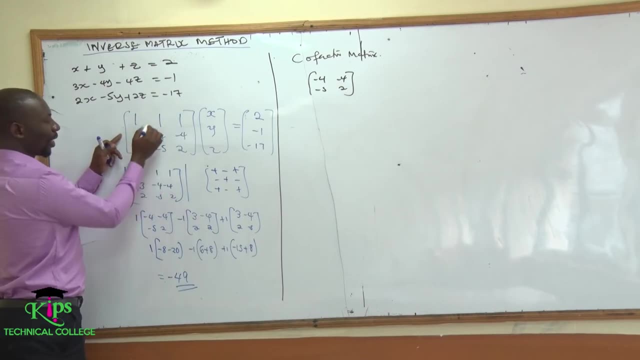 Remain with negative five. two from your two by two matrix. You start at this point, you close this row and this column. you remain with this two by two matrix. So the second one. you start at this point, you close the row and column. 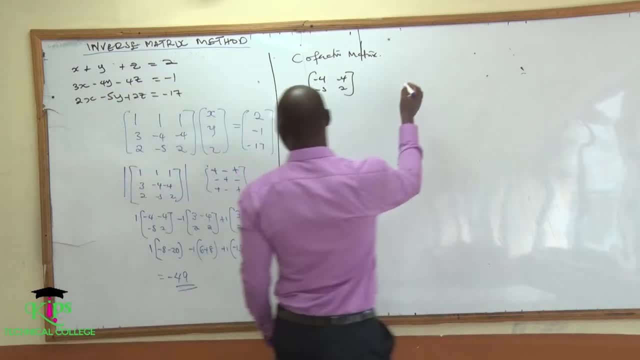 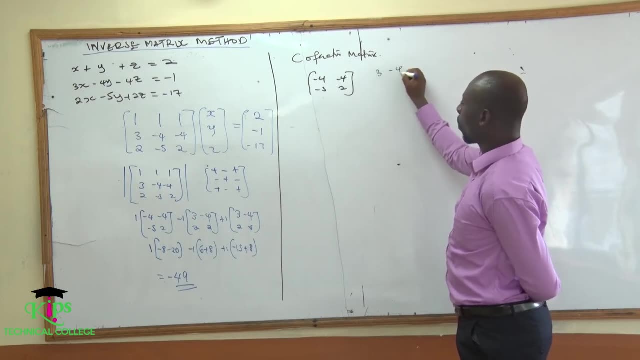 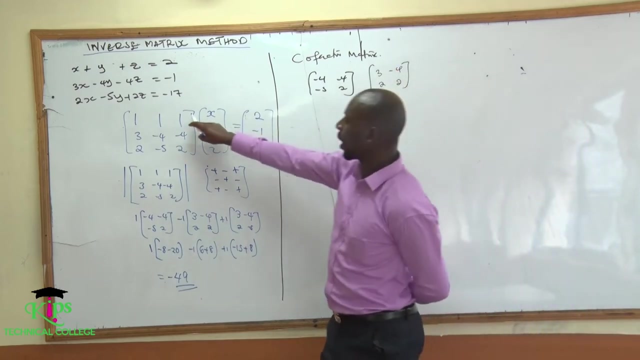 you remain with this one and this one, this and this. So you remain with: let's do it. you remain with three negative four, then two and two as your two by two matrix, Then the third term, that is one. you close the row and column where one is. 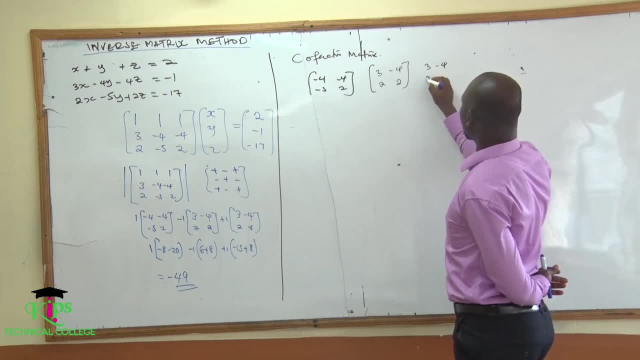 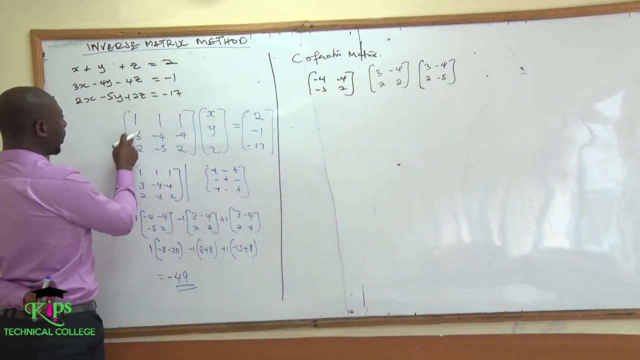 that one. you end up with three negative four, two negative five Negative five in that format. Then you come to the second, the middle row, that is at three. you close this row and the middle column, you do it: one one negative, five negative two. 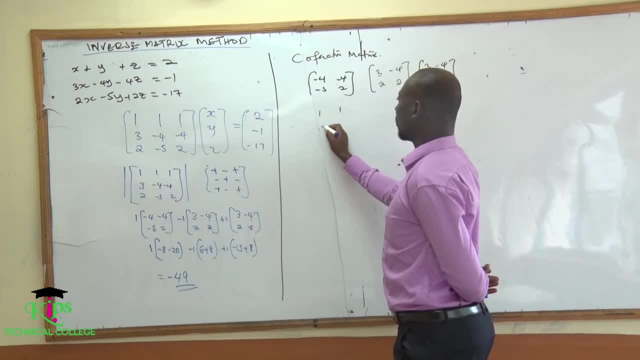 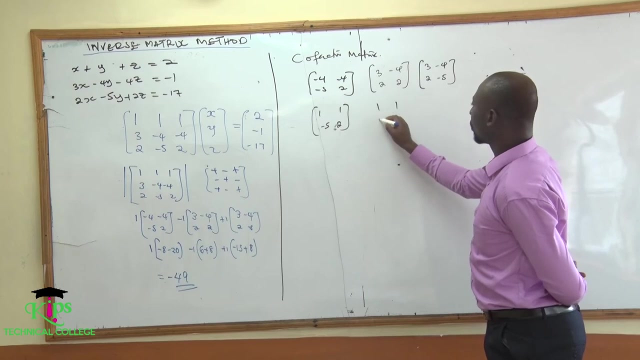 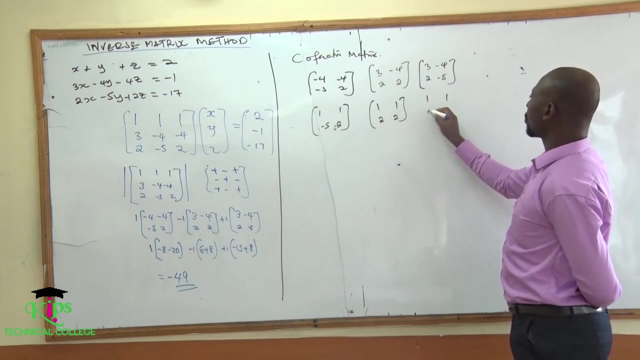 So that one shall be one, one negative five negative negative five, two. Then the second one that is at point of negative four. you end up with one, one, two. The third at negative four. you end up with one, one, two negative five. 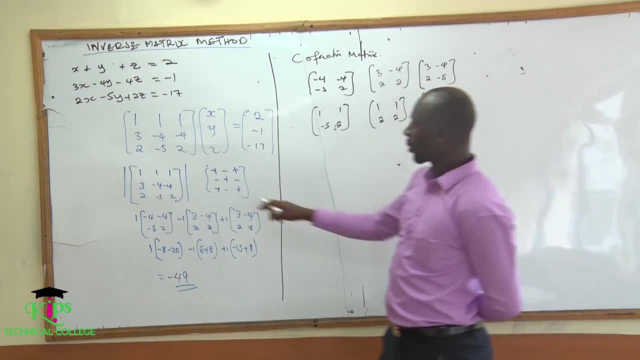 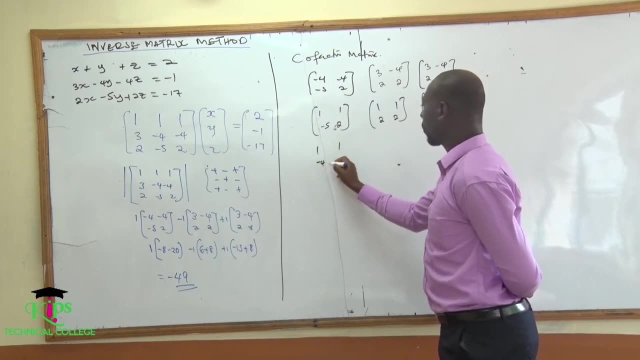 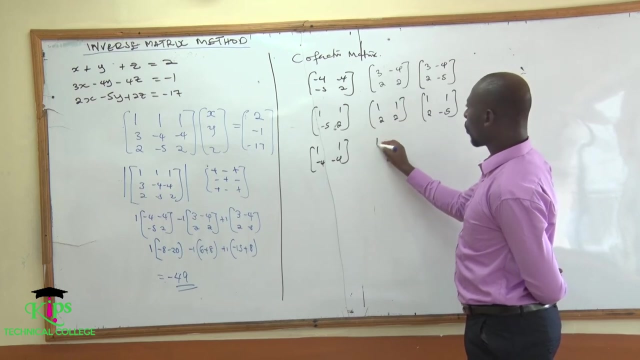 At the linear point, that is, at point two, you close the row and column, you end up with one one: negative four, negative four. Then at the negative five, you close the row and column, you end up with one one, three, negative four. 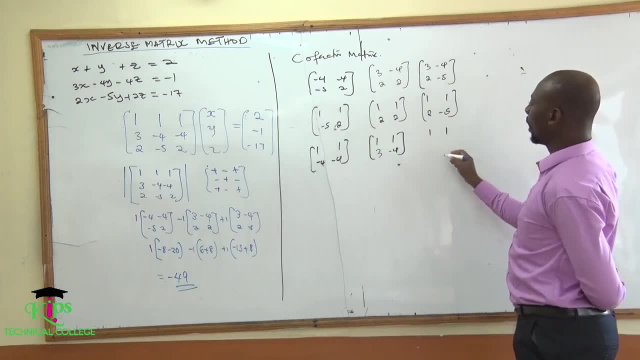 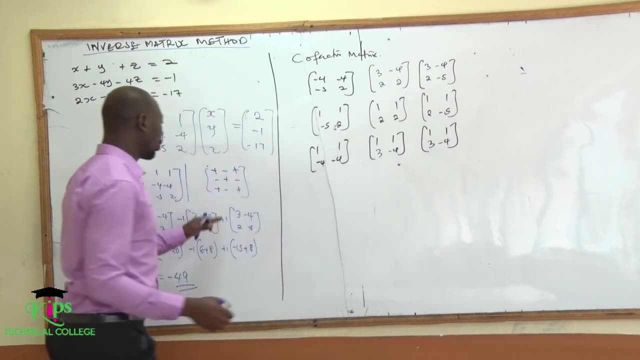 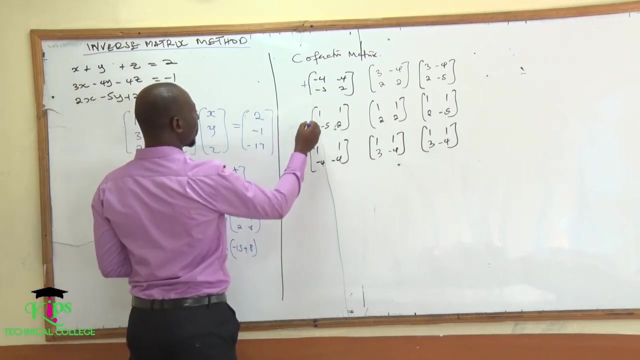 At point two you end up with one, one, three, negative, four in that format. Then, after forming the two by two arrays, in each bracket you introduce the two, the signs. So the first one you give each sign, this one is positive, negative, positive. 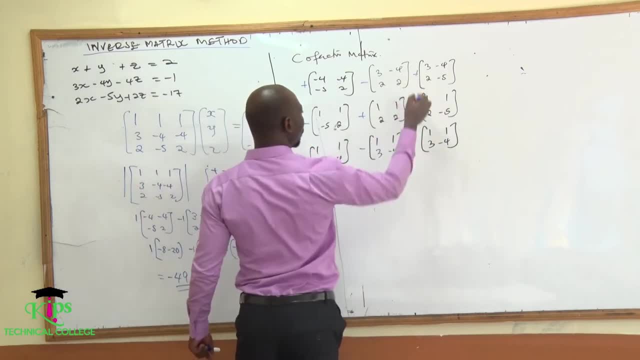 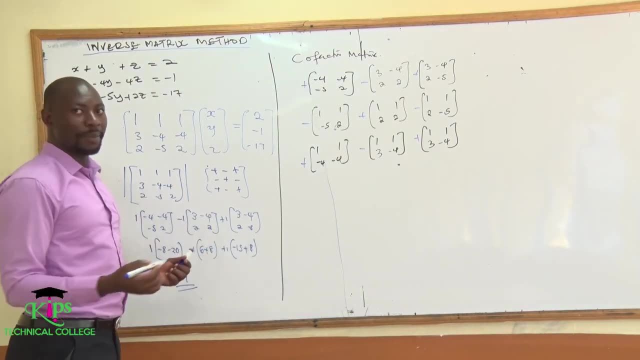 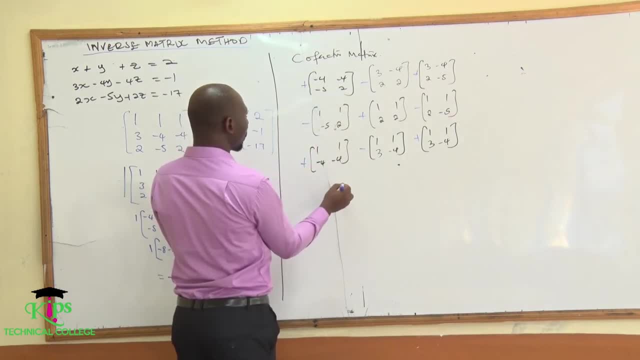 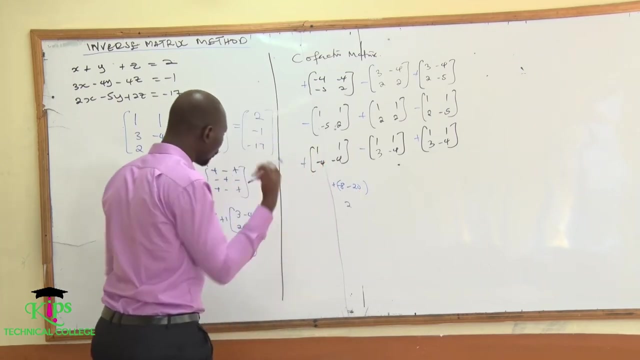 two by negative, four by two, that is eight negative eight minus twenty with a positive sign at that point, Then at this point you end up with two by one. by two is two, five by negative negative. five by one gives you negative five. 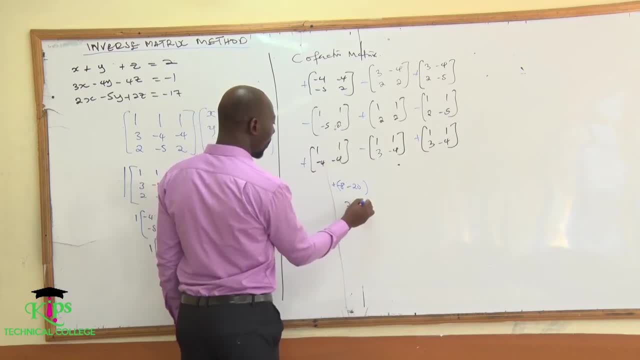 So this is two minus five becomes plus five. But you multiply by a negative sign outside. At this point is two by one, by negative four, that is negative four, Then negative four by this one becomes, then it adds up with a positive sign outside. 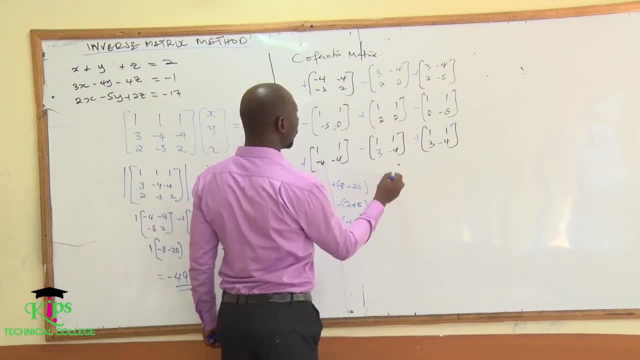 Then in this column is negative, that is two by three, that is six Negative, eight negative and negative becomes positive. Then the positive sign: two by two, two by one is two, two by one is two minus two. in that format: 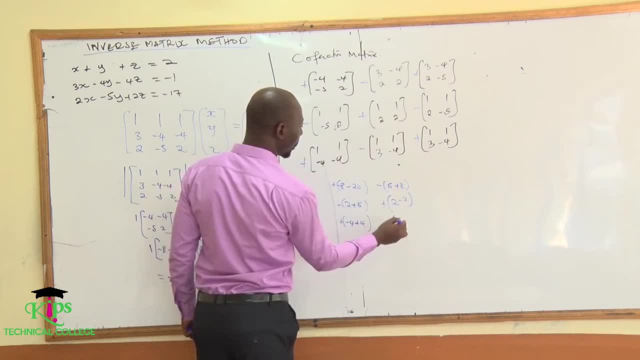 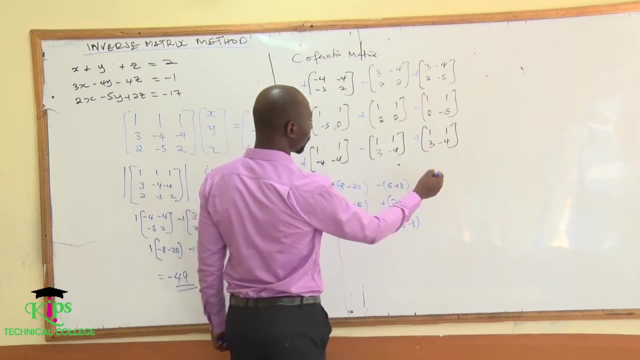 With a negative sign here: two, one by negative, four is negative. four, Three by three, one is negative is three. then minus three. That format last row, that is three by negative, five, that is negative. fifteen, Two by negative, four is negative four. 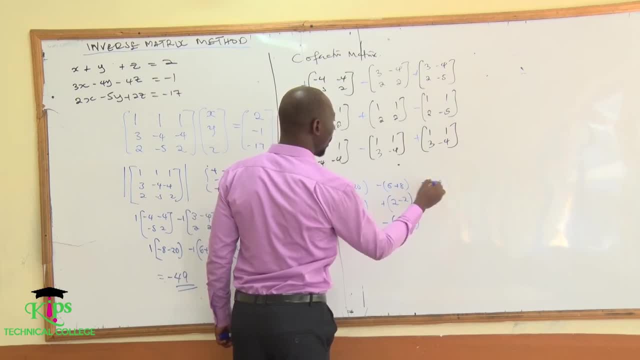 Then the positive and negative and negative gives it a positive sign And the positive sign outside Negative into two by one, by negative five is negative five. Two by one is two, Then that is less two. That format positive sign outside. 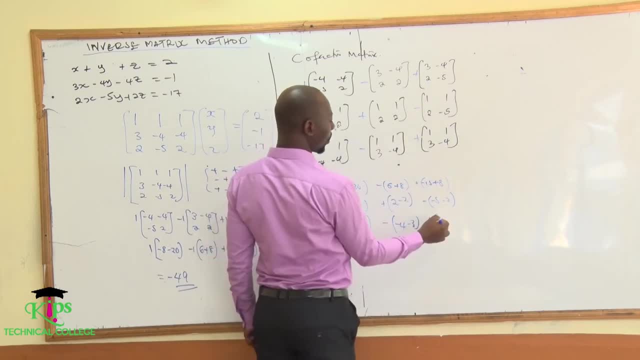 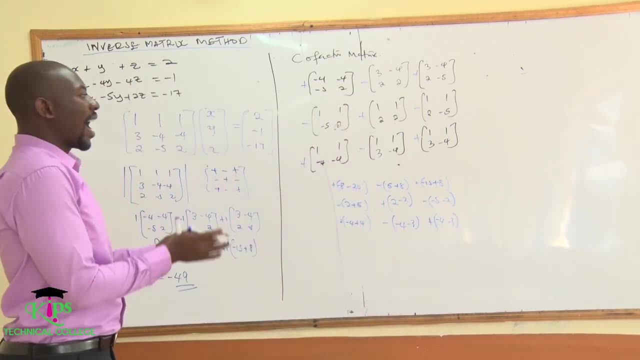 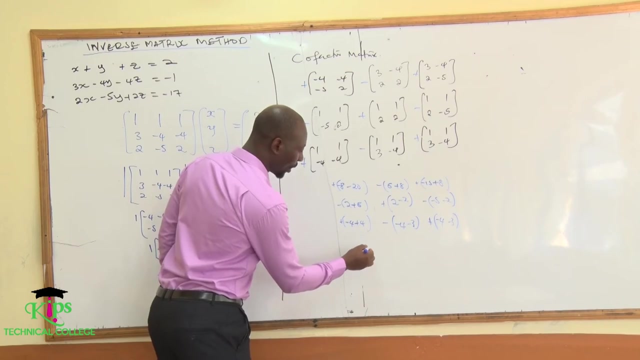 In the preceding format. one by negative four is negative four. Three by one is three minus. So you solve each un-bracket for you to be able to form a condensed three by three matrix, That one shall be. we shall have negative twenty-eight in this one. 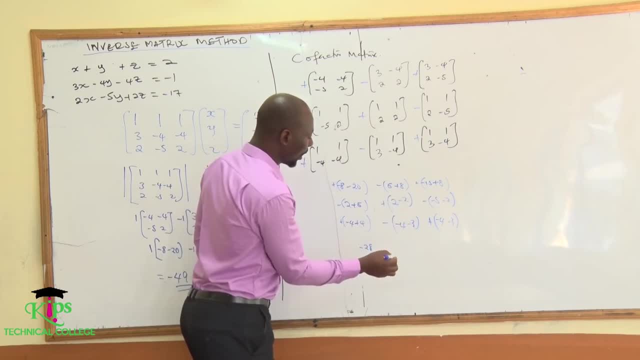 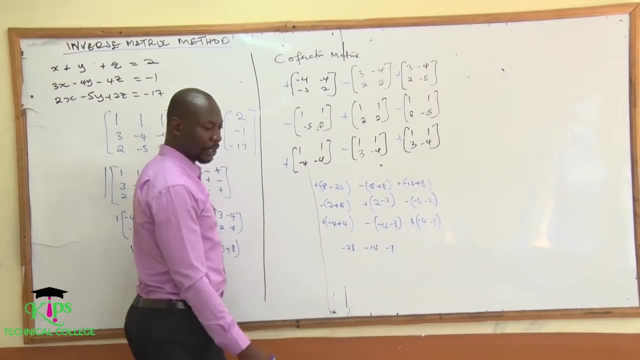 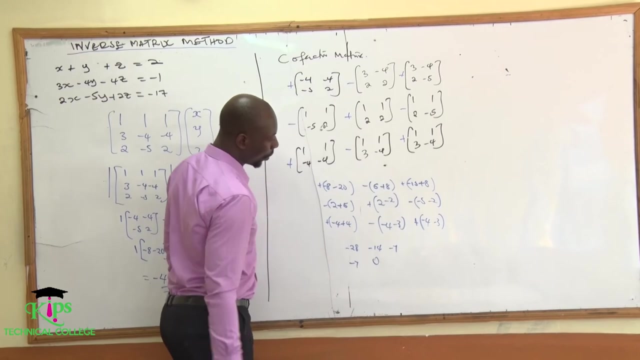 The second one, that is this one. you have end up with negative fourteen. Then we have this one: gives you negative seven. You proceed. This one also gives you negative seven. The middle term gives you zero, That is two by two. 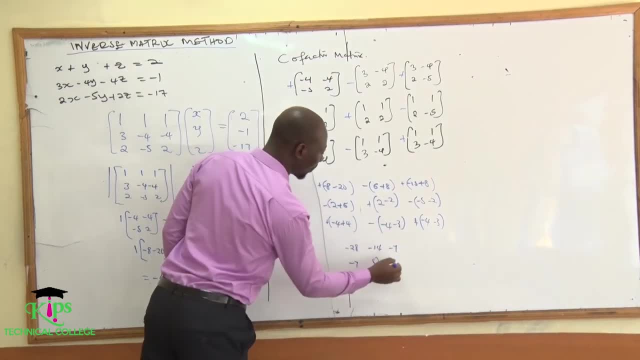 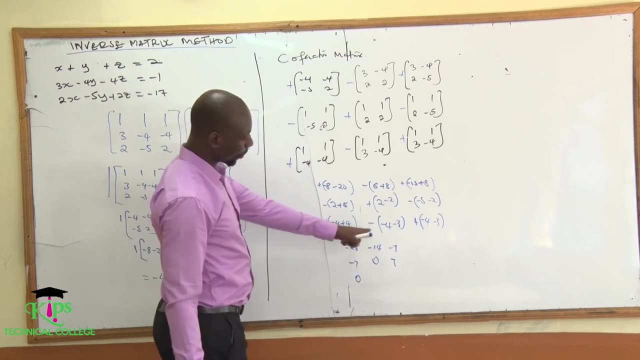 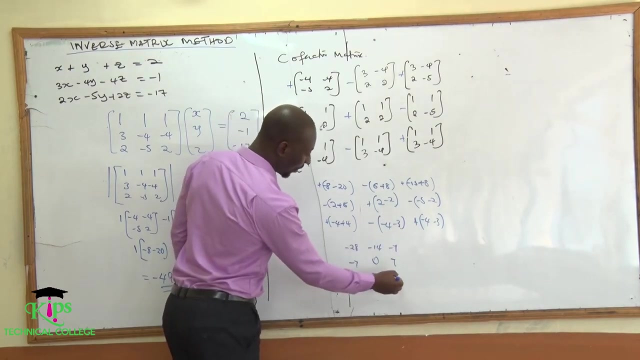 This is negative five minus five. That is negative seven Times. the positive sign gives you positive seven outside, Then this one is positive four And negative four gives you zero. Then this is negative seven times negative outside gives you positive seven, Then the last term is negative seven. 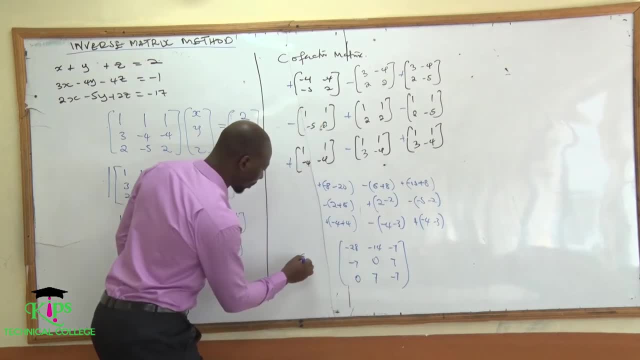 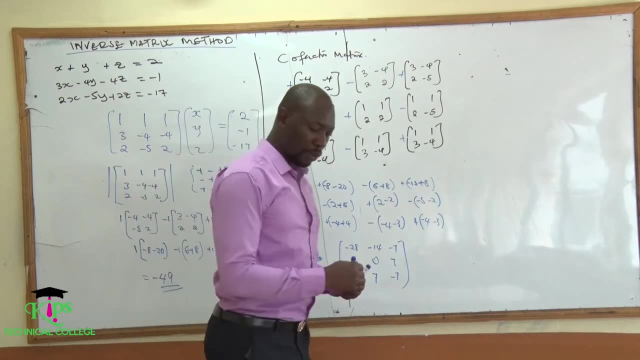 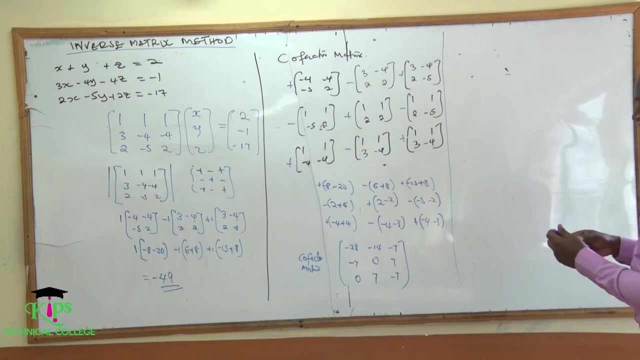 So this is what we call the cofactor matrix. So we need to get what we call the adjoint To get the adjoint of a three by three matrix. what we transpose to get the adjoint, Transpose, transpose to obtain the adjoint. 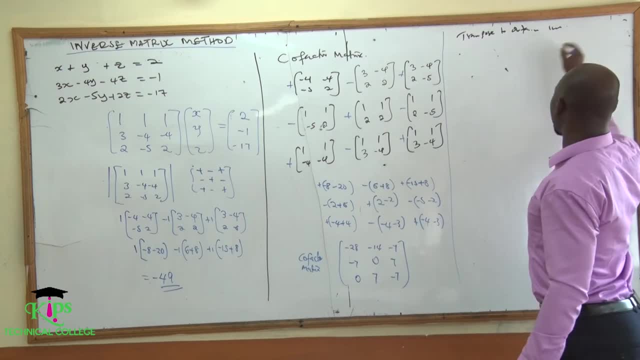 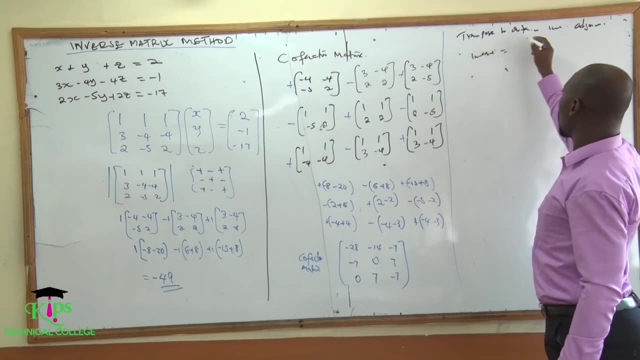 So if you transpose, you change the rows of the ad column to get the adjoint. After getting the adjoint then the inverse of the matrix inverse is given as one over the determinant, One over the determinant times the adjoint. So we take one over our determinant. 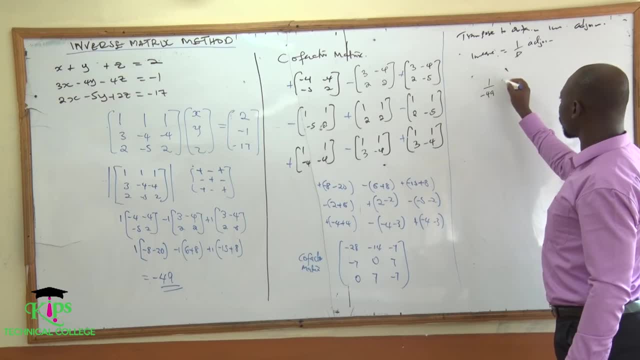 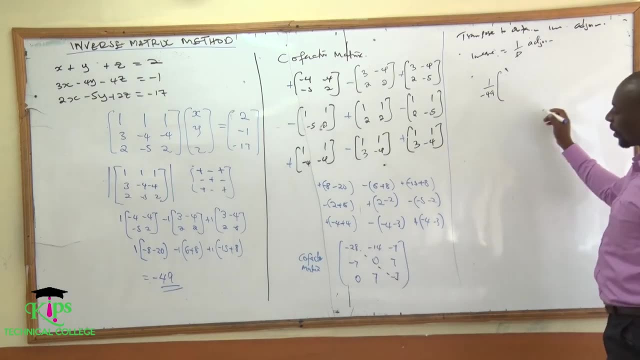 That is one over negative forty-nine. Then we multiply by the adjoint To get the adjoint. you take it this way: You maintain the first horizontal column, That one shall be negative twenty-eight, Then zero, Then at here we have got negative seven. 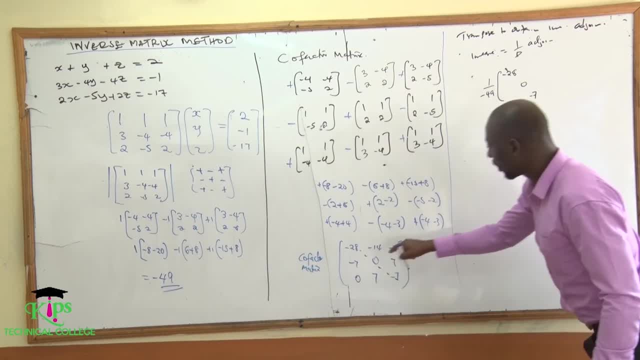 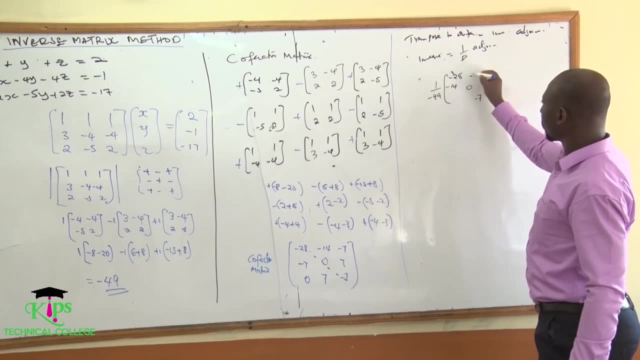 That one is maintained, Then you reverse this one and this one. Here we increase that to negative. fourteen Comes here. negative seventeen come here. That is negative fourteen here. Here negative seven. Here we have got zero. Comes here. negative seven goes down. 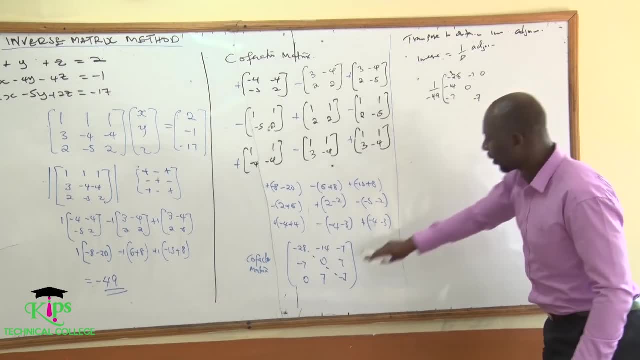 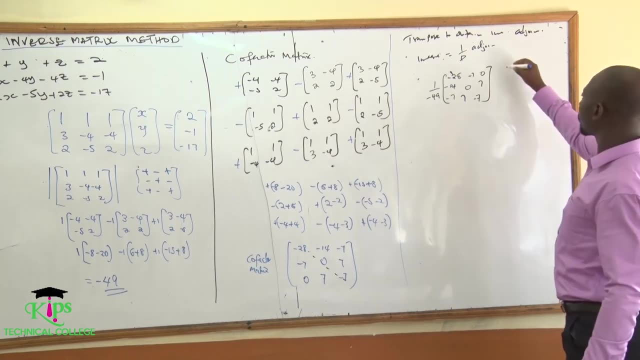 So here is negative seven, Here we have a zero And the term this seven and seven, crosses terms, So it is just seven, seven. So that is our inverse, So this is the inverse Inverse of the matrix. So what we do? we take the inverse and multiply both sides. 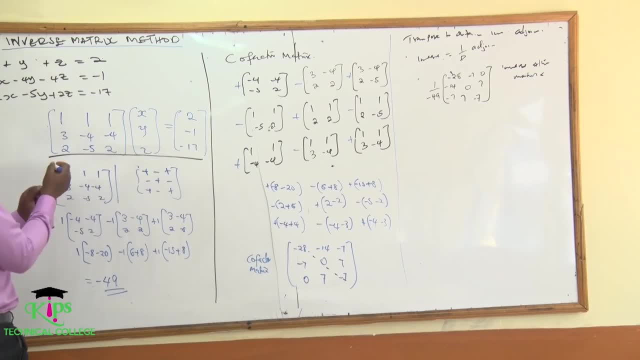 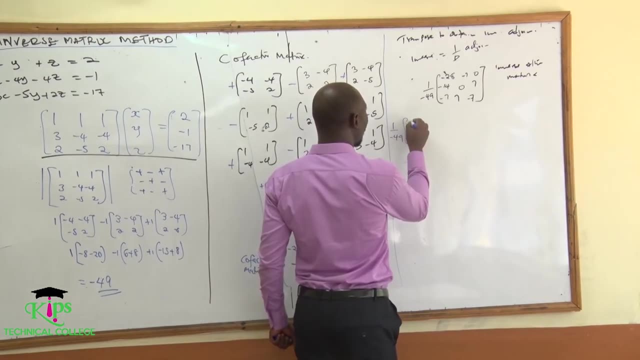 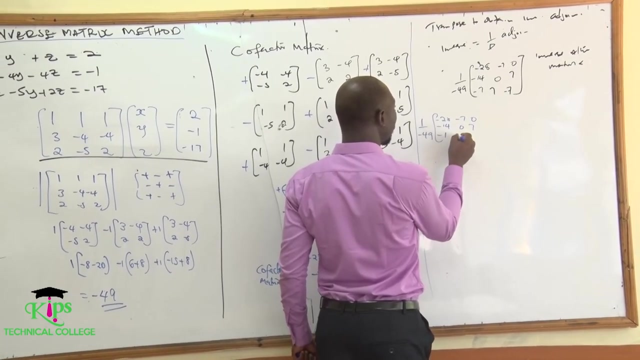 We go to the original equation: Multiply both sides by the inverse, That one shall be. you take our inverse, That is one over negative forty-nine Into negative twenty-eight. Negative seven: zero. Negative fourteen, zero seven. Negative seven, seven seven. 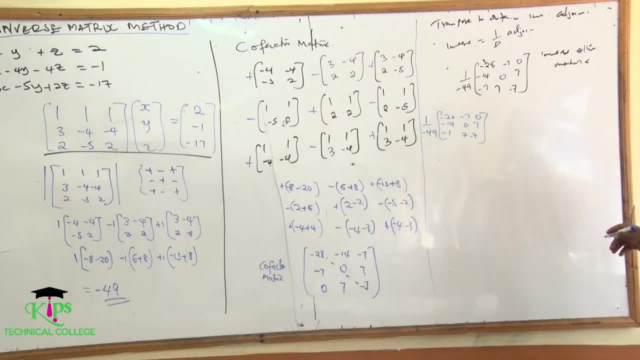 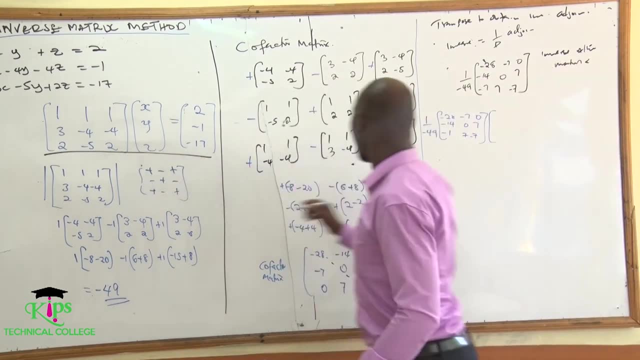 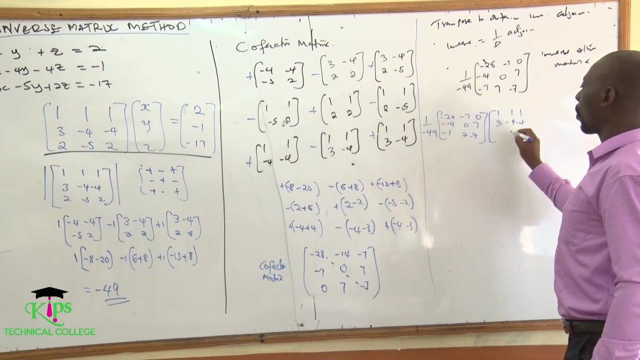 Negative seven. in that format. You take it in that format. Then you multiply by the original matrix, which was this side, That is this one. That is one, one, one, Three negative four Negative four, Then two negative five, two. 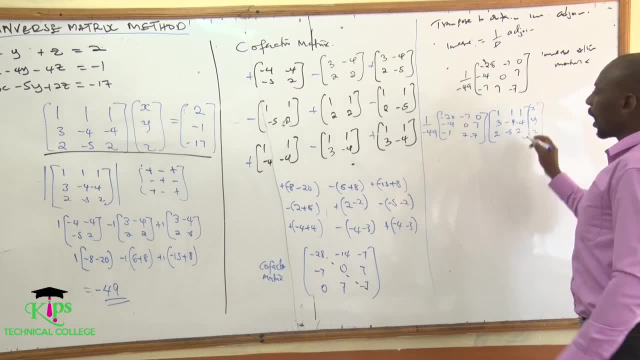 X, Y and Z, And whatever you multiply on the left, you also multiply on the right. That is one over negative forty-nine Into the matrix that is negative twenty-eight, Negative seven, zero, Negative fourteen, zero, seven. Then negative one, seven, negative seven. 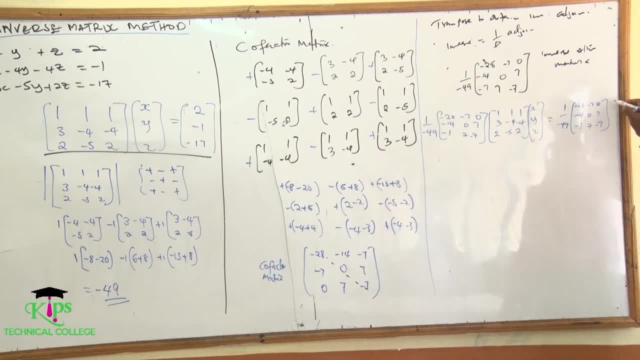 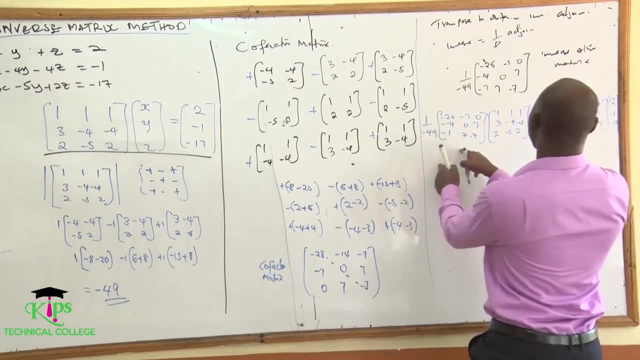 You multiply by what was on the right, That is, two negative, one negative, seventeen. So you multiply by that, So you multiply both sides. So this one is the inverse of this matrix, Any number. For example, if you have a number N, 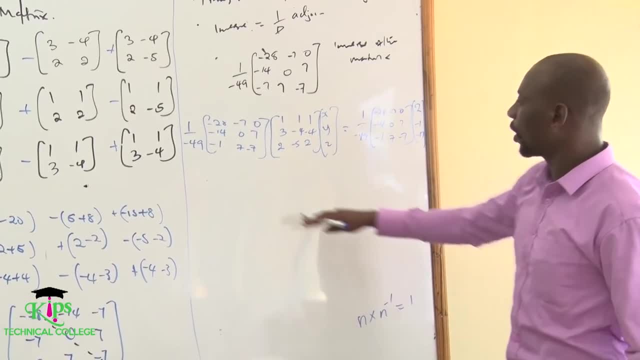 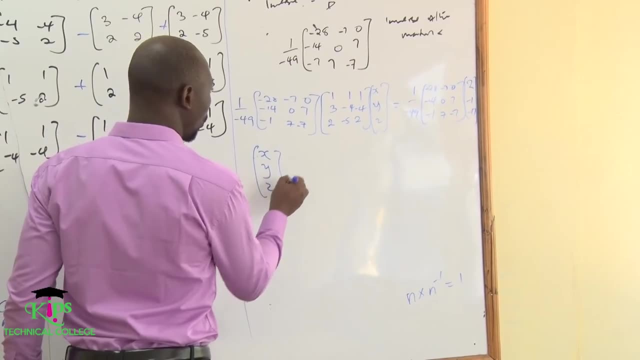 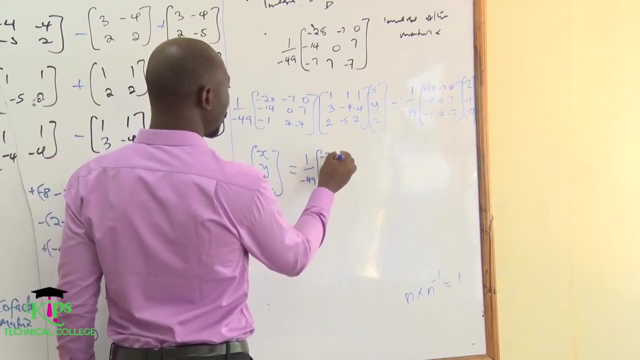 If you multiply by N- it is inverse- You shall get one. So this side automatically gives you one. So it means that this side means X, Y and Z is equal to that other side, That is, one over negative forty-nine Into negative twenty-eight. 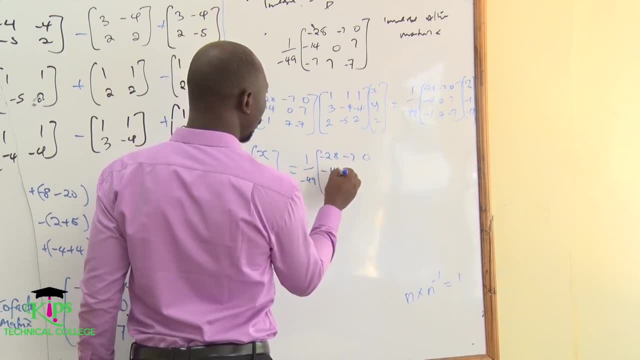 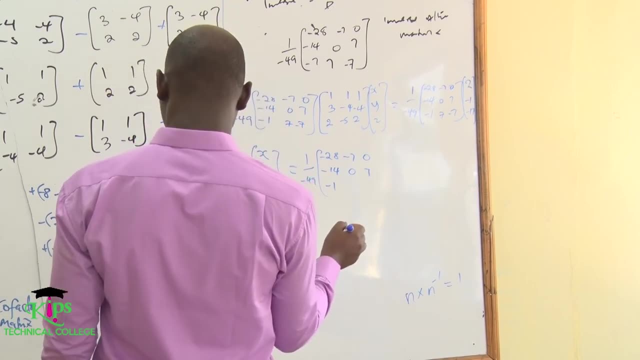 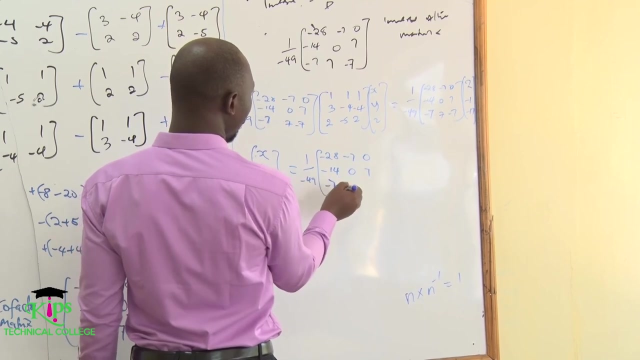 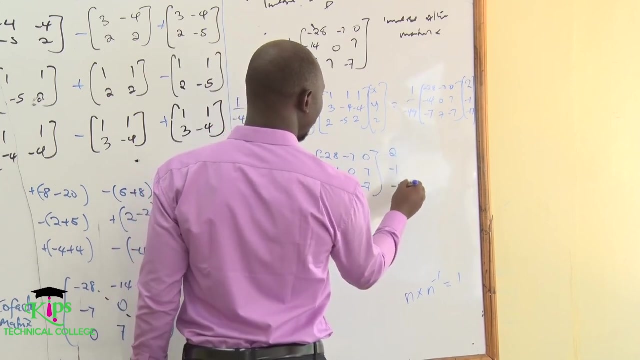 Negative seven: zero. Negative fourteen, zero, seven. Negative seven, That is negative seven. This one is negative seven. Negative seven, seven, negative seven. In that format: Multiply by two negative, one, negative, seventeen. So if you multiply the two, 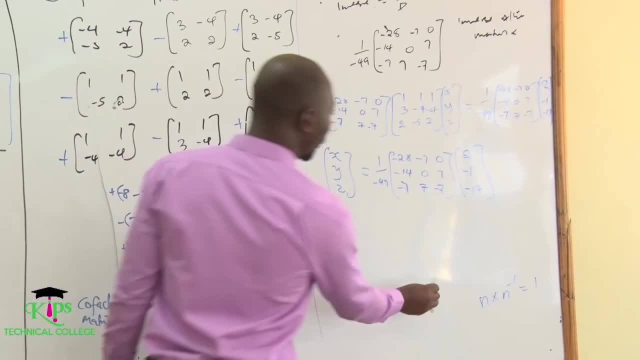 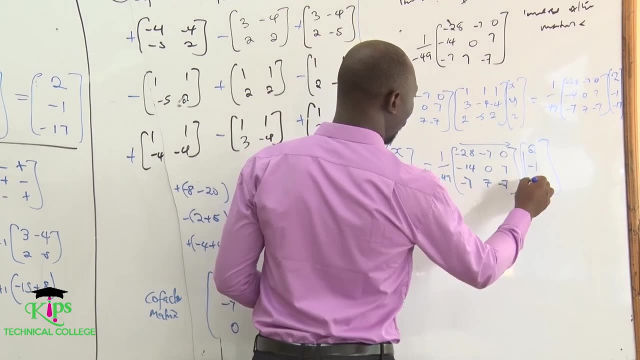 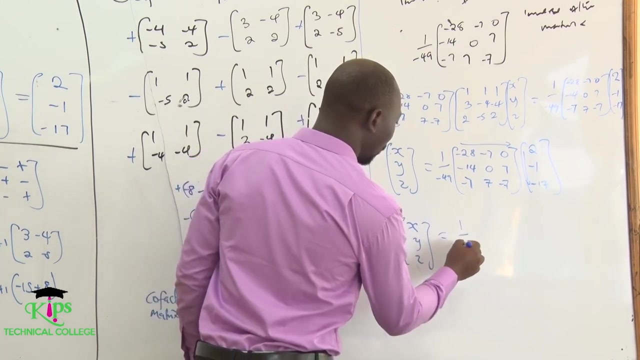 Remember how we have done: how to multiply three by matrices, That is, rows and columns, Rows by a column, Then you add them together. X, Y, Z shall be therefore equal to one over negative forty-nine Into, If you multiply all this row and this column and sums together. 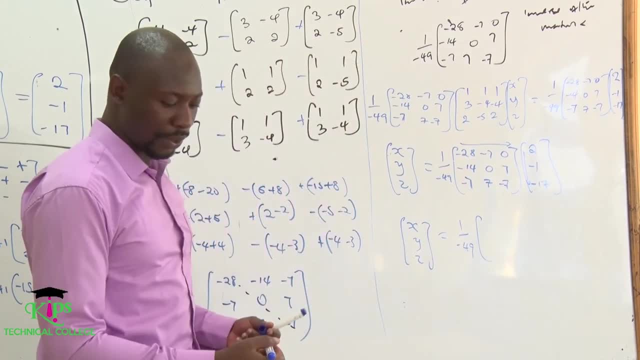 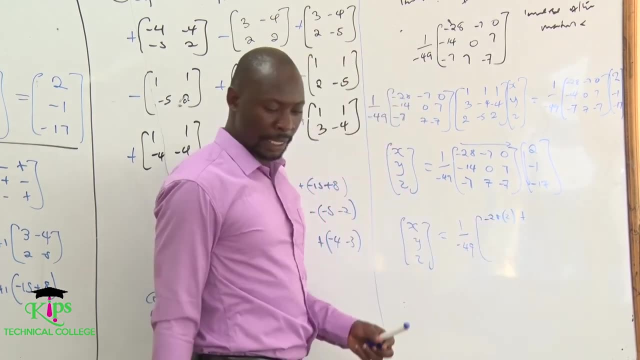 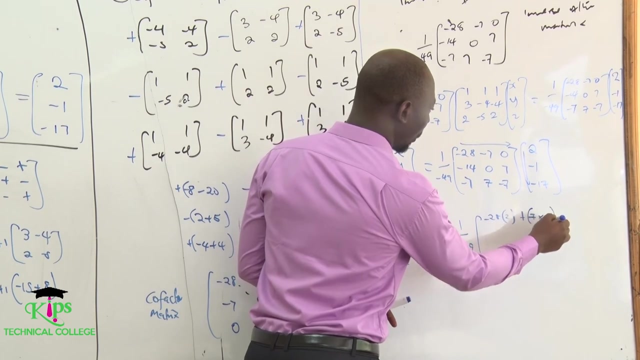 You get negative. Okay, Let's just do it together. If you multiply the rows and together you get negative. twenty-eight into two Plus That is negative seven by negative two. Negative seven by negative one, Then zero by negative. seventeen Into negative seventeen. 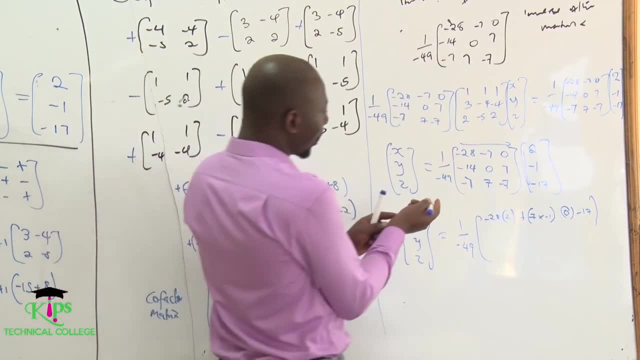 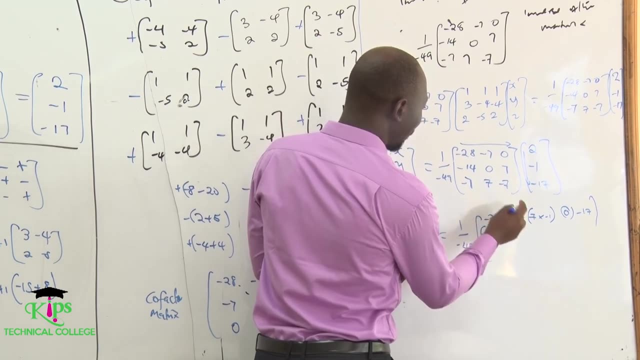 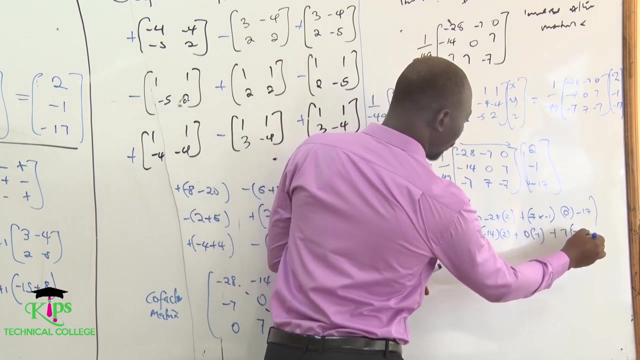 That gives you the upper line. Then the second one shall be negative fourteen by negative two By two, sorry By two Plus zero by negative one Plus seven By negative seventeen. Then the last column, That is negative seven into two. 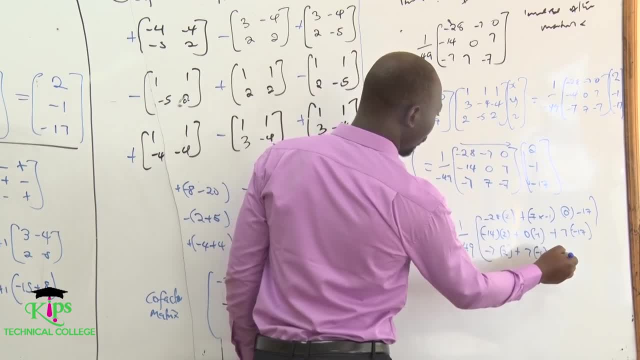 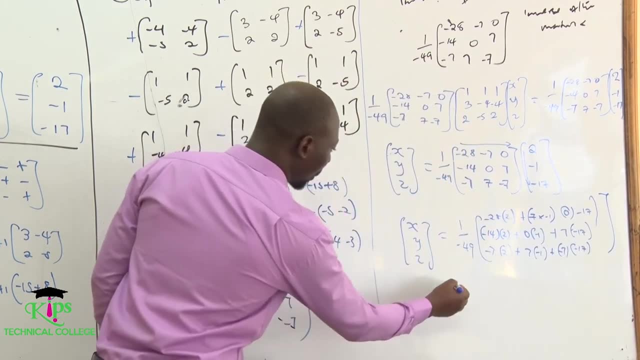 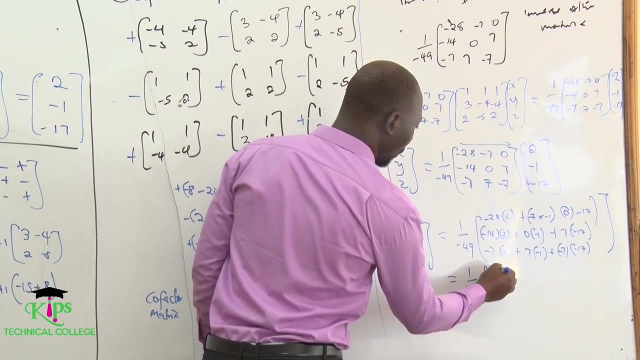 Plus seven into negative one, Then only plus negative seven Into negative seventeen, So that one shall give you The matrices that you intend to get. That one gives you One over negative forty-nine Is equal to The upper one. if you sum you get negative forty-nine.